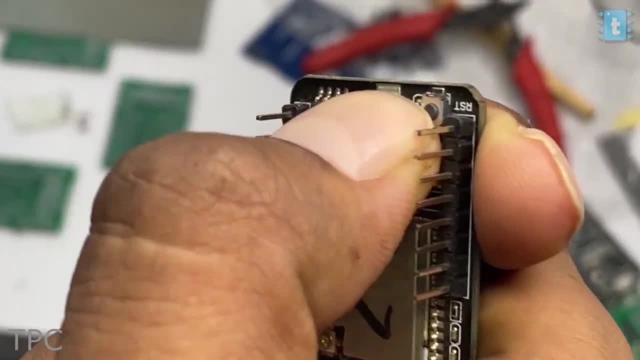 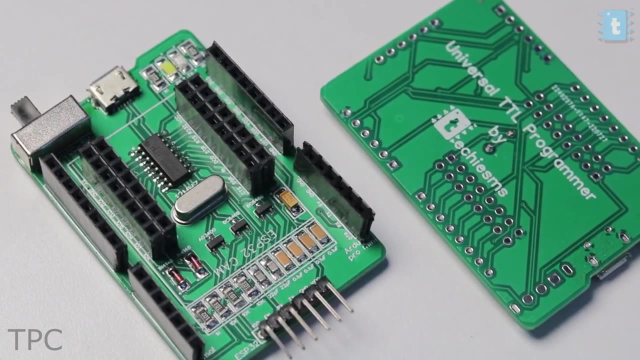 because we have to press the reset button, which is provided on the back side of the board. To make this process easier, Techie SMS built this ESP32 programmer. We just need to insert the ESP32CAM into the programmer, connect it to the USB. 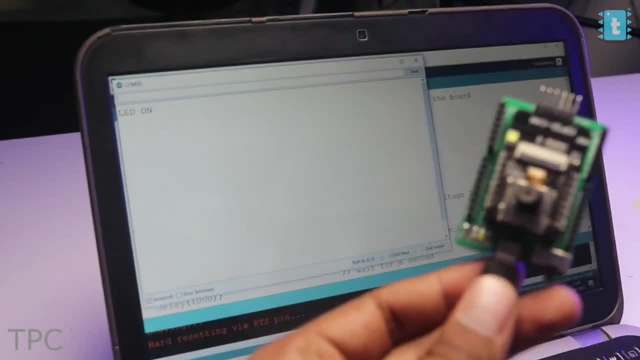 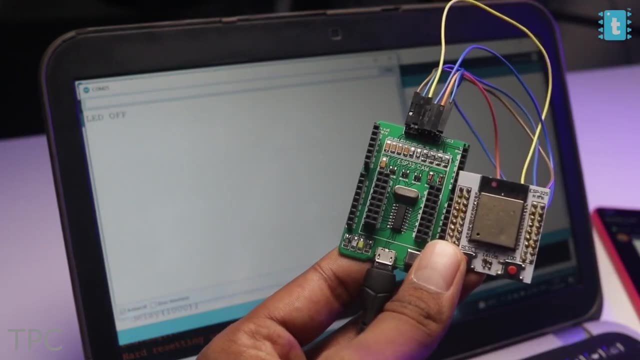 upload the code and voila, The ESP32CAM is programmed without the need to press the reset button. Apart from the ESP32CAM, we can also program other boards like ESP32Chip and Arduino Pro Mini without removing or adding any components from the programmer. 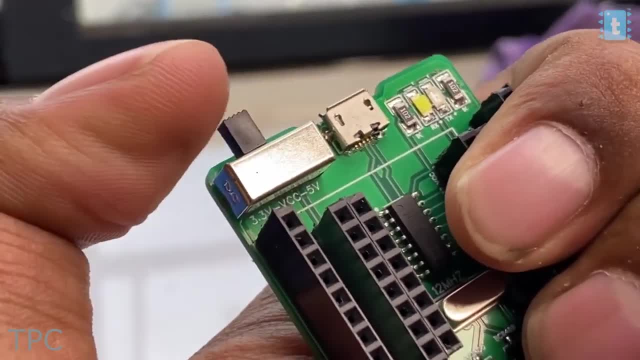 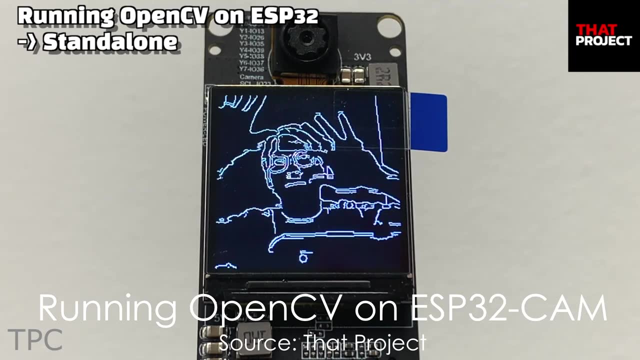 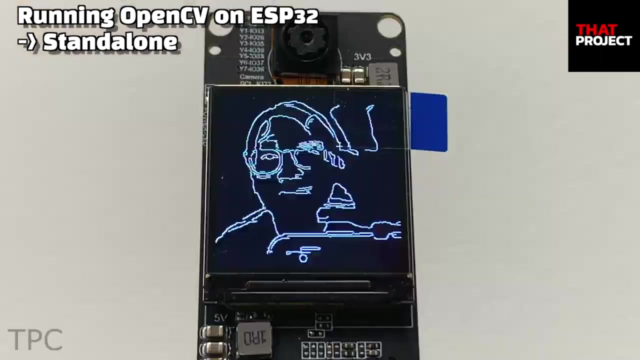 This board's compatible to work in 3.3V logic as well as 5V logic Number 9.. Running OpenCV on an ESP32CAM is not that easy, but by following this project you can do it. The ESP32CAM captures the image and uses canny edge detection with the OpenCV. 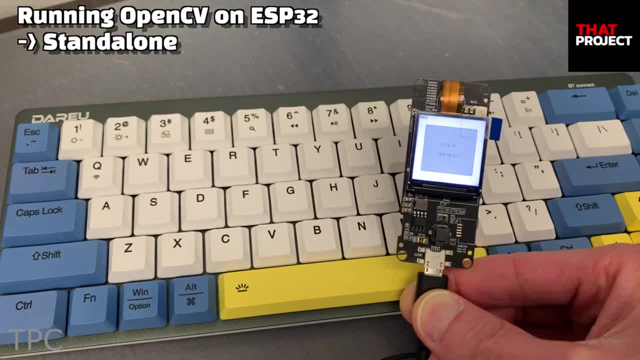 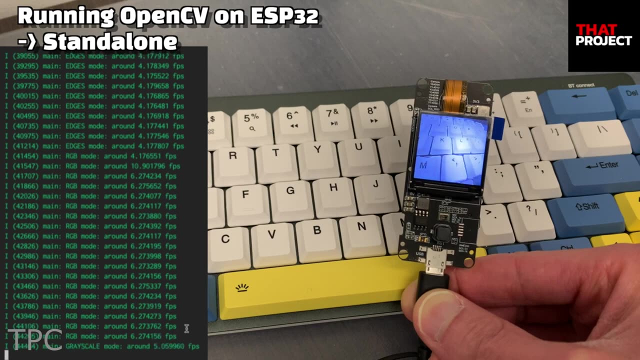 library in real time. Once the code runs, the screen displays the TTGO demo for three seconds. After that, RGB mode, scale mode, binarized mode and edge mode are executed repeatedly. The canny edge detection requires the most computational power, Hence the FPS of the 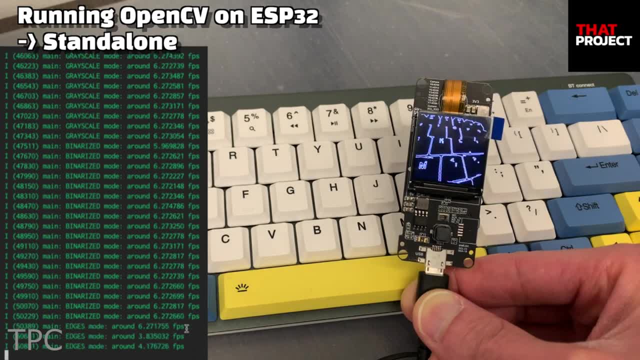 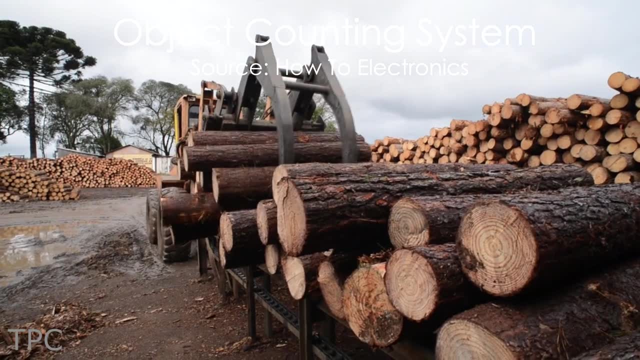 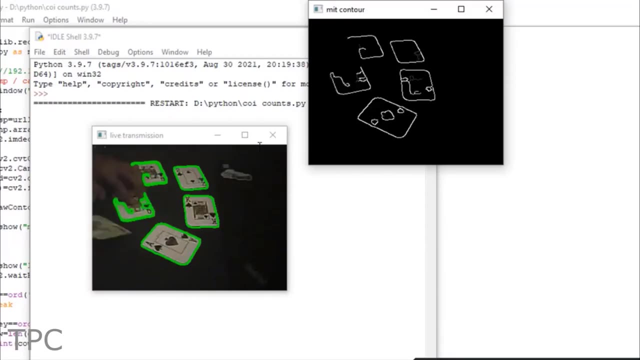 displayed image is low, but on average it displays the image with 6 frames per second. Number 8.. Counting some limited objects is easy, but if the number's too large then you may definitely need some help. For that this little project can be of great use. To detect the object it uses a step-by-step 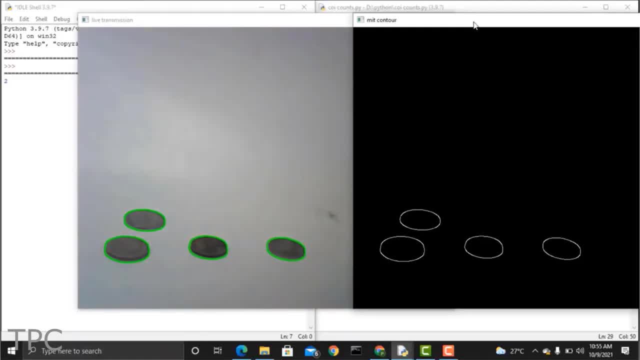 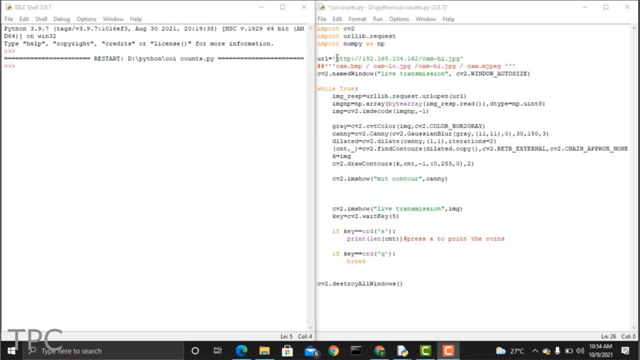 method of entering and exiting the image. If you're using a computer, you can use the image or frame conversion. Initially, the RGB image is converted to grayscale so that the color contrast is visible and mathematical operations can be performed easily. After that, the image 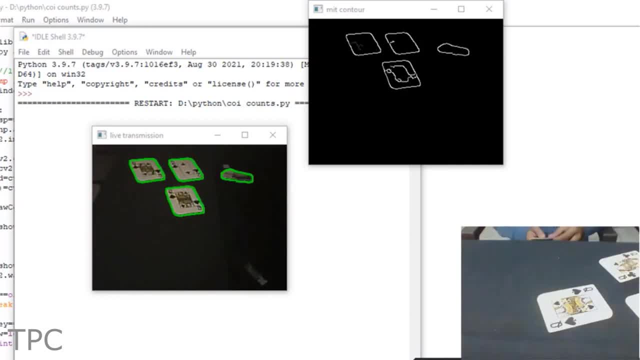 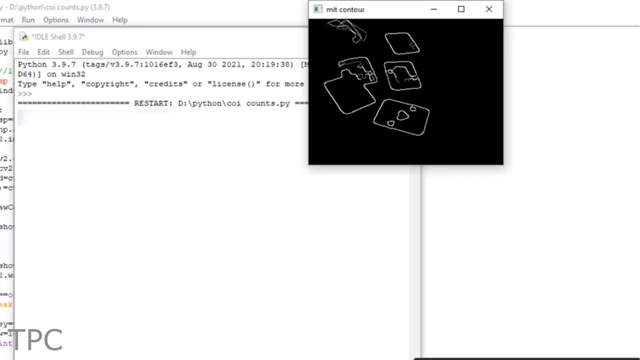 is blurred to blend the colors and, using canny edge detection, the edges are detected. Finally, to properly join the detected edges, the image is dilated. In this way, the number of closed figures is detected and printed on the serial monitor. 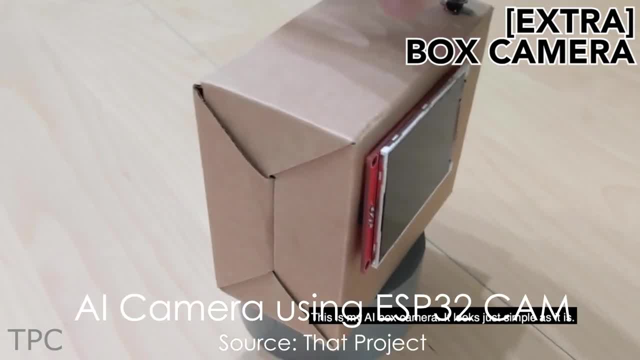 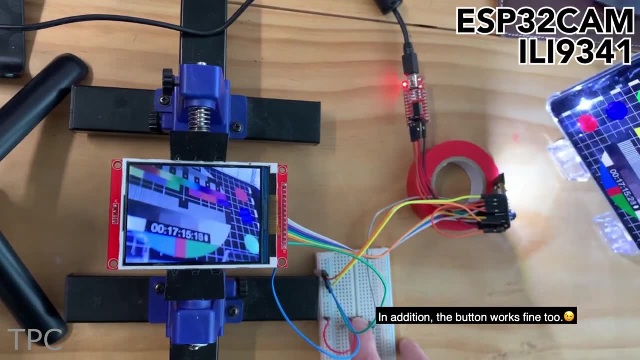 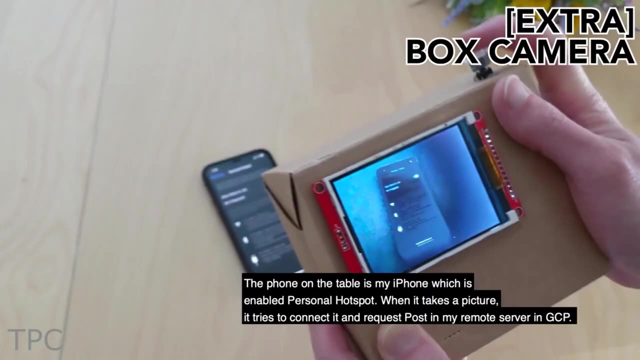 Number 7.. If you want to make your own AI camera, then make sure to try this project. Eric placed an ESP32 cam inside a cardboard box, a push button to capture the image and a screen to view the captured image. But how does it tell the object details? So first the ESP32 cam captures the image. 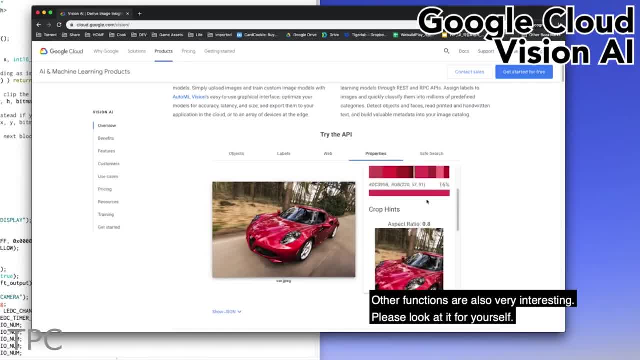 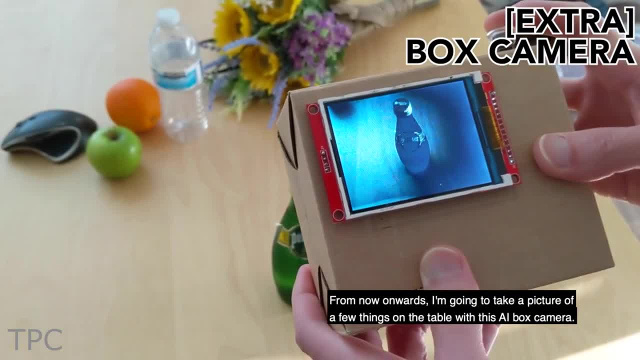 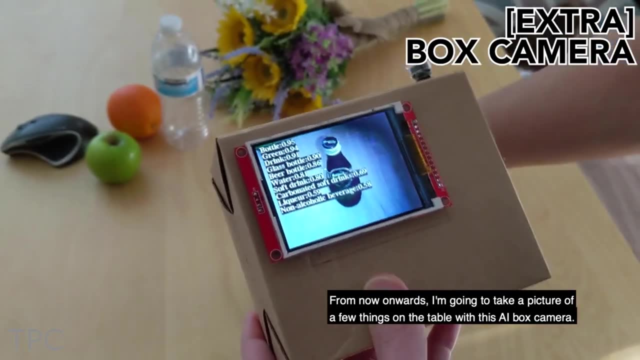 and uploads it to the Nodejs server. It then calls the Google Vision API to get an image annotation. Once the object's identified, the image is returned to the ESP32 cam via the same process And with that you can get the details of any object that you want. 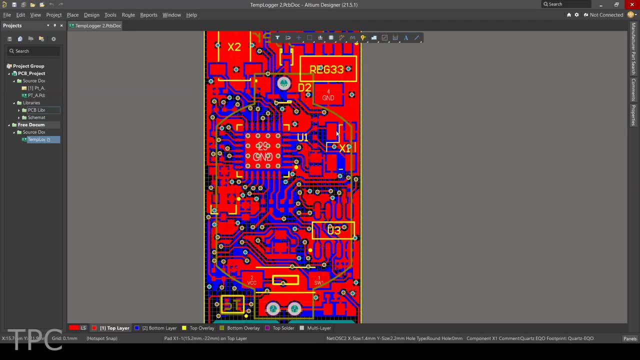 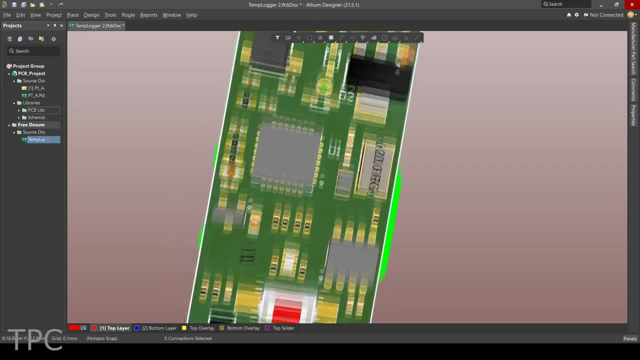 Altium's a PCB design software that's both powerful and easy to use. With its intuitive interface and comprehensive set of features, Altium Designer makes it easy to create high quality PCB designs, And with all-new Altium 365, now you can share your PCB designs with. 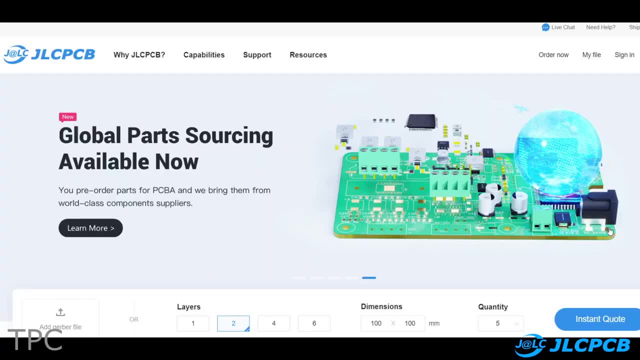 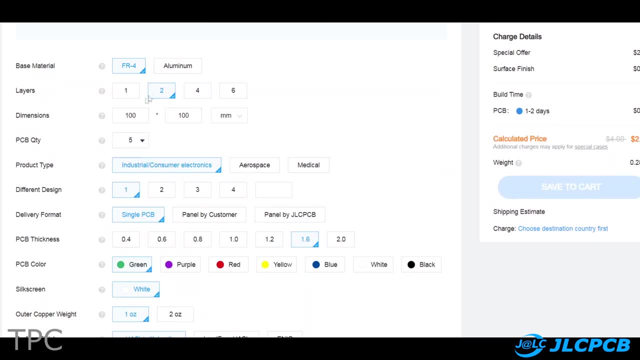 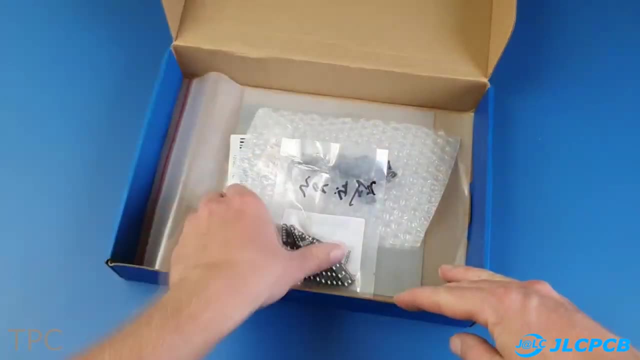 anyone from anywhere with a single click. And to convert these designs to real-life PCB boards, look no further than JLCPCB. They provide all types of PCB services and assembly at very competitive prices. Their high-quality PCBs, quick delivery and great customer service make them the 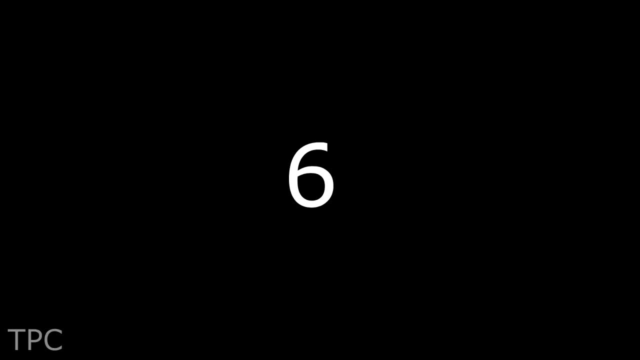 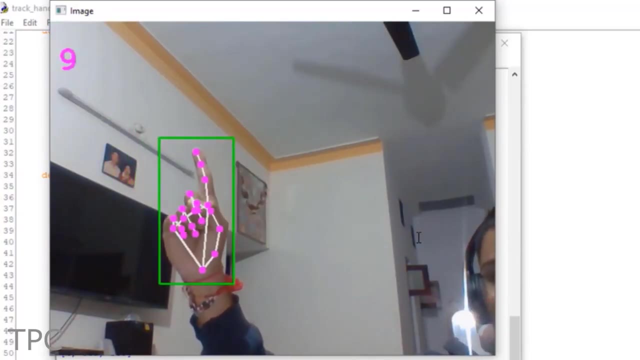 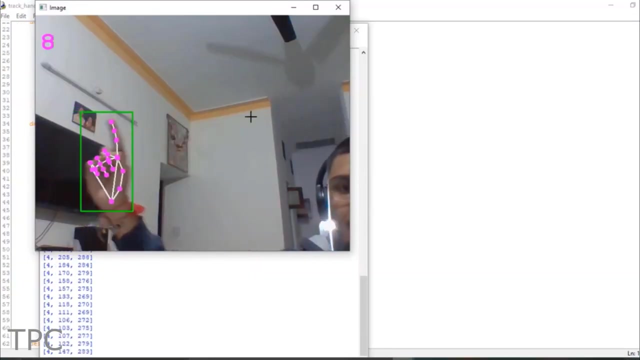 perfect partner for your electronics projects. Number six: Using this project, you'll be able to detect hands and fingers using Python and implement it to use as a gesture-controlled virtual mouse. In this demo code, using a webcam, we can see how image recognition's working. Using your index finger, the cursor can be moved in. 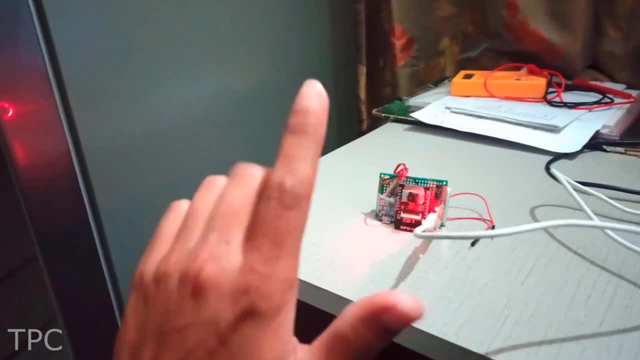 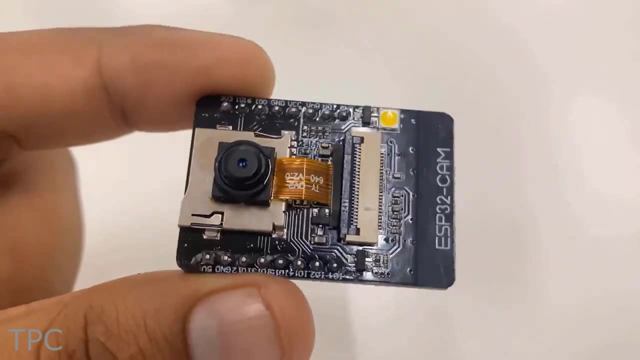 any direction. To click on any particular location, the middle fingers move downwards, while keeping the index finger upwards. To use it using an ESP32 cam, you'll only need to modify the dimensions and frame rates in the code. All other things will remain the same. 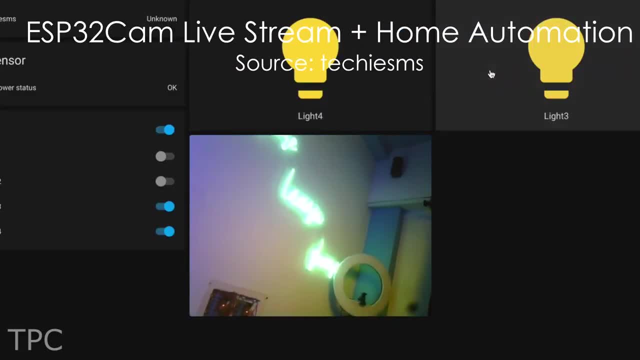 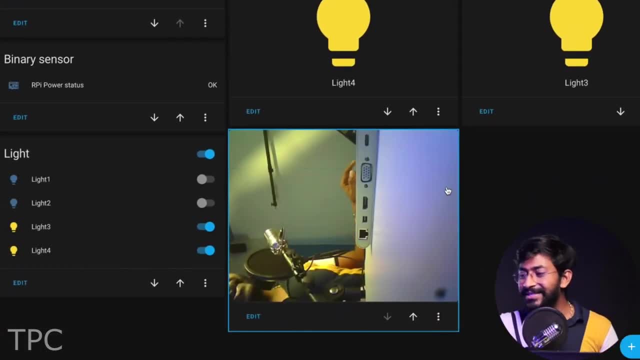 Number five: If you're looking to fully automate your home using a single dashboard, then this project will help you. Using this project, you'll learn how to stream a live video on a home assistant platform. This means you'll want to use it every day, so you'll need a good 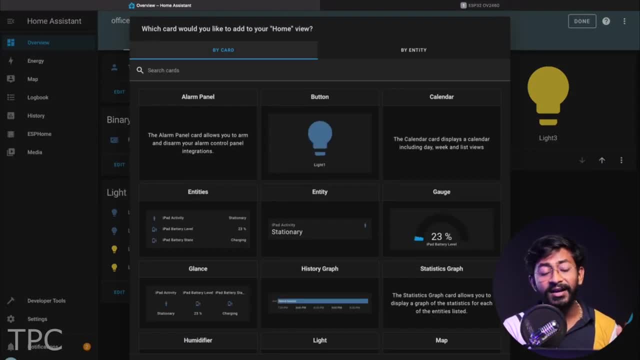 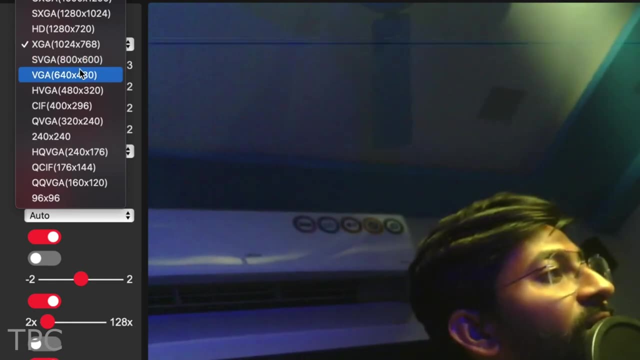 platform, as well as control the status of various devices using the same platform. The stream starts to lag if a higher resolution is selected, so try to keep the resolution low. The dashboard runs on a local area network, so make sure to connect each device to the same network. 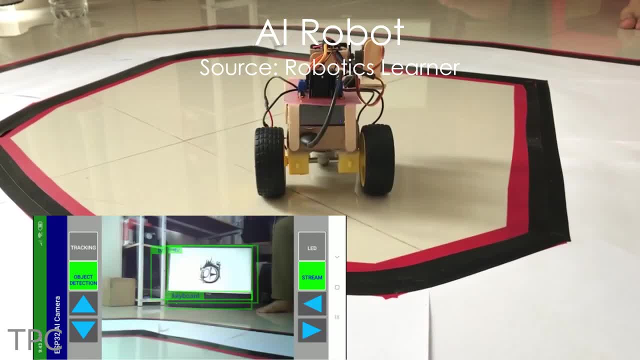 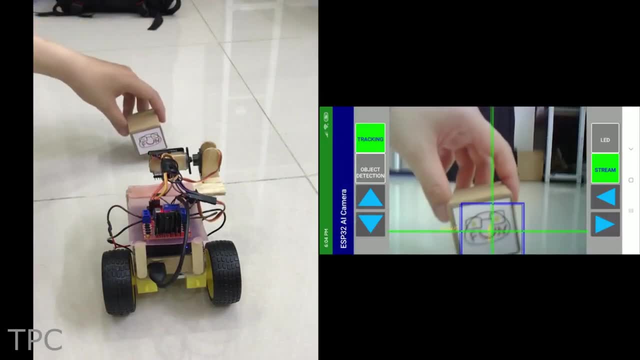 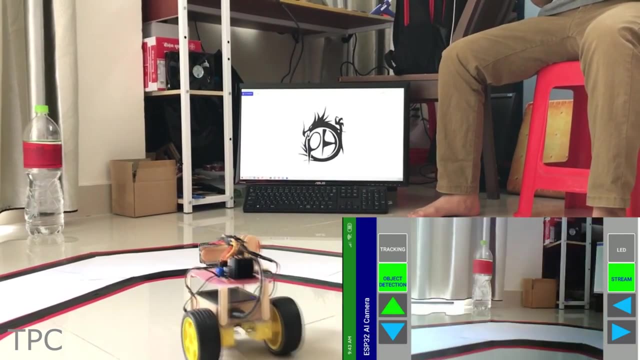 4.. If you're trying to make an intelligent robot, then make sure to try this project. This robot not only moves in a specified lane, but can detect and track objects pretty easily. The robot's controlled using an Android application. The ESP32 cam streams the. 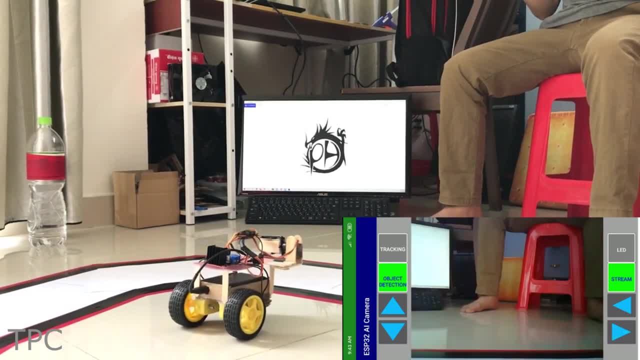 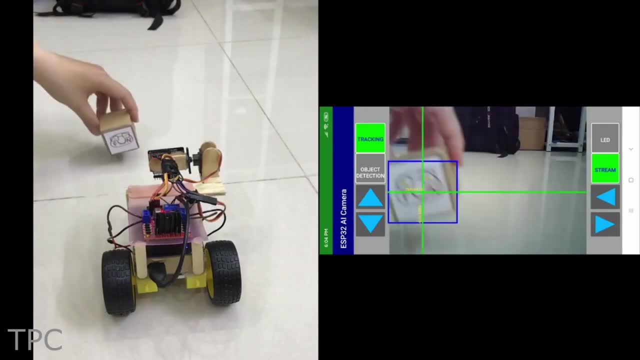 video to the application, and the image processing part's done there only. It detects objects at a high speed and low latency. The pan and tilt movement of the camera's provided using a servo motor. Currently, the chassis of the robot's made using cardboard and sticks. 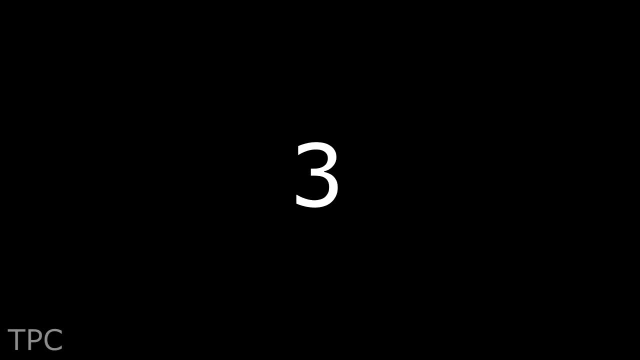 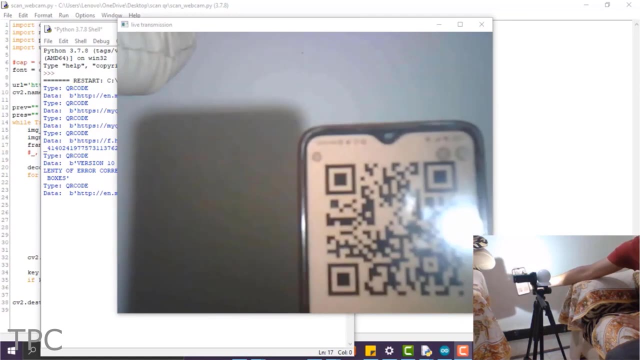 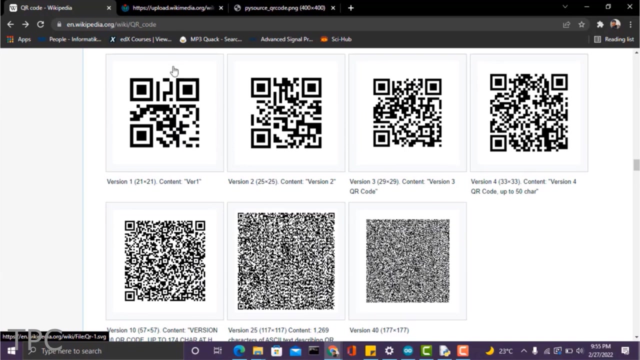 but it could be updated using a metal one. 3. With this project, you'll learn how to make a QR code scanner using the ESP32CAM module in OpenCV. Based on the amount of information a QR code can store, different versions of QR codes are available. 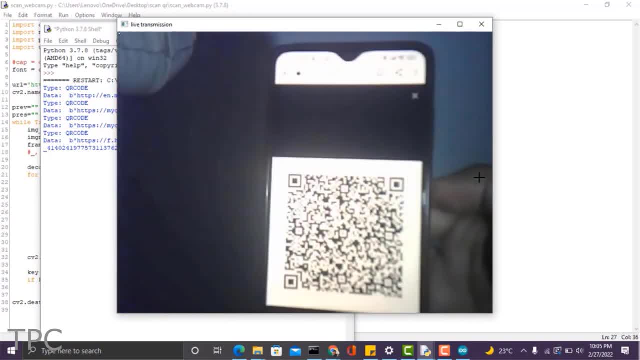 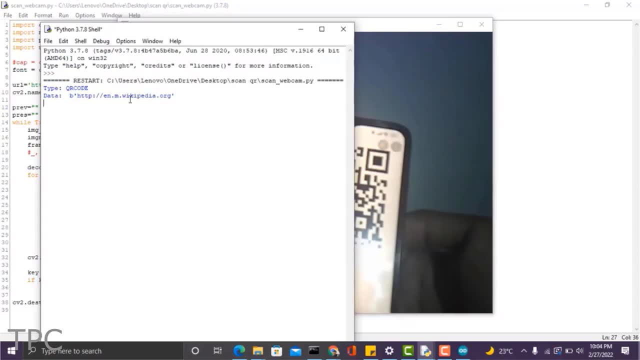 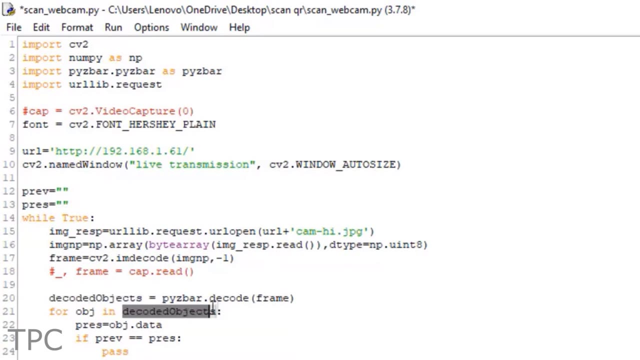 Using this project, even complex QR codes can be decoded. To decode any QR code, you'll need a Python library. The code extracts the frames from ESP32CAM and decodes the data using a library function. The decoded data is then printed on the screen. 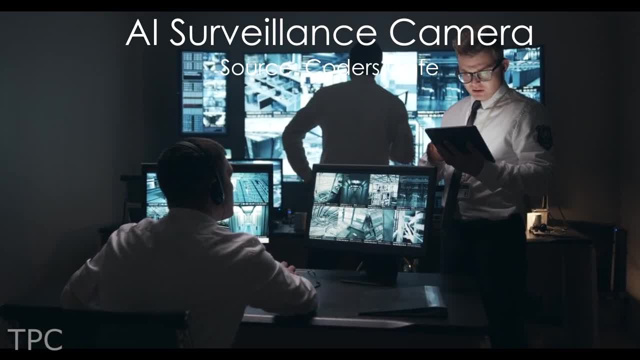 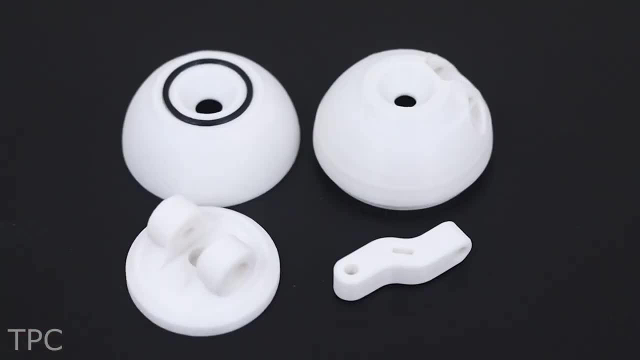 2. Are you looking for a surveillance project at a very low price? Then, under $10, you can make a surveillance camera using an ESP32CAM and a 3D-printed frame. The camera itself detects the movement and does not require a PIR sensor. 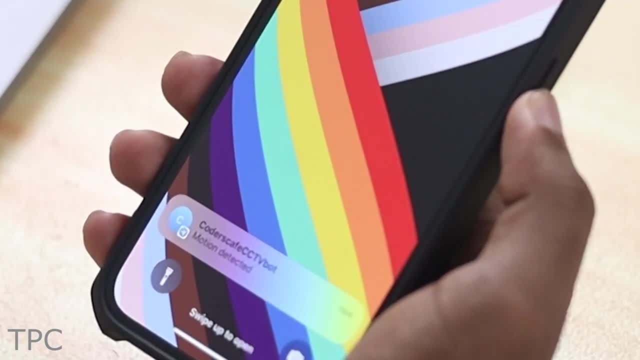 As the motion is detected, it notifies you with a message on the telegram application. 3. As the motion is detected, it notifies you with a message on the telegram application And if you have an Internet connection, you can use the ESP32CAM module to send the video to the ESP32CAM module. And if you have an Internet connection, you can use the ESP32CAM module to send the video to the ESP32CAM module. And if you have an Internet connection, you can use the ESP32CAM module to send the video to the ESP32CAM module. 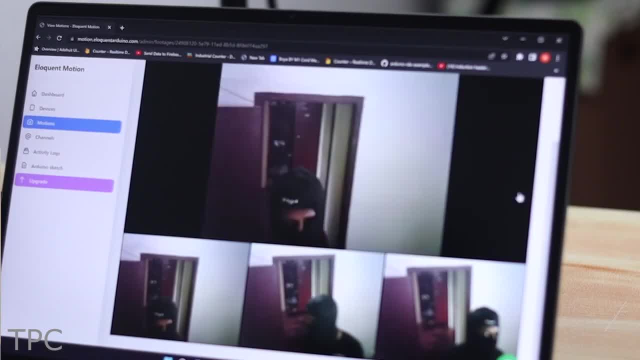 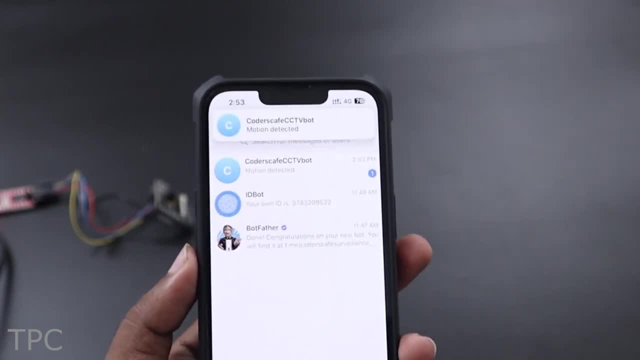 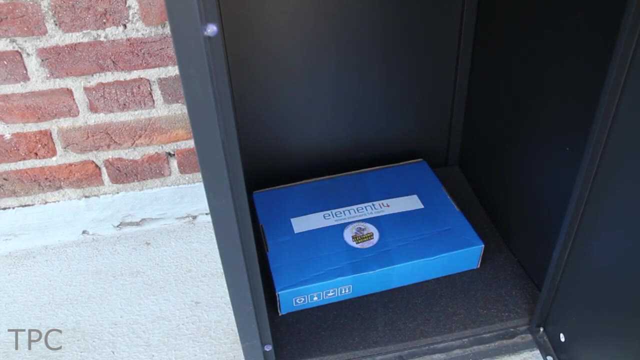 And if you have an Internet connection, you can view the images and short footage of the intruder from anywhere and take necessary actions. With this project, your premises are secured, and that, too, on a limited budget. 1. Sometimes it becomes frustrating while waiting for a mail or any parcel that you've ordered. 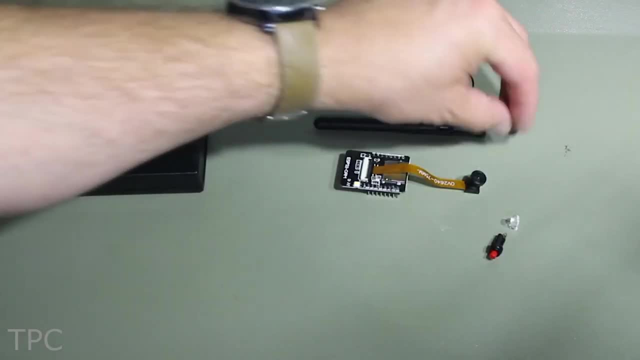 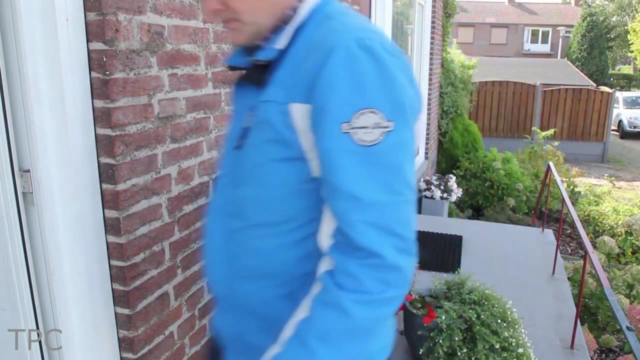 and checking your mailbox again and again is not a practical option. In that case, you can use this mail monitoring system. As any package is dropped into your mailbox, a switch gets triggered. An ESP32CAM module will take a photo of the package. 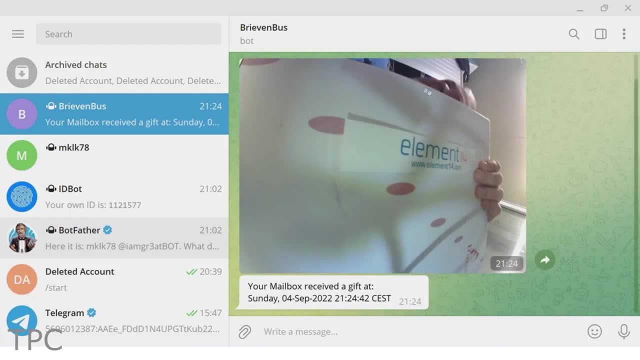 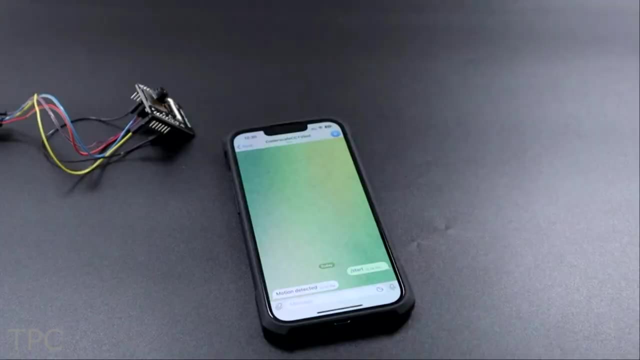 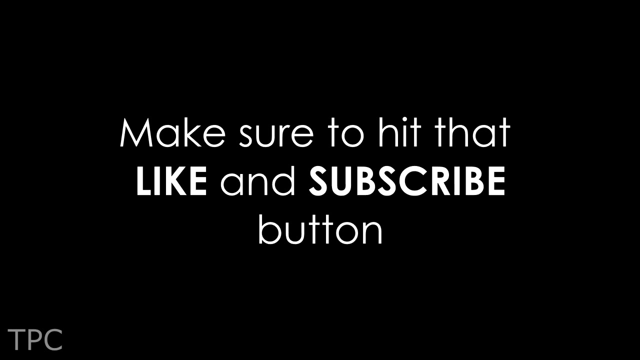 and that photo will be sent directly to your telegram messenger. The resolution of the picture is fine, which will aid you in distinguishing which parcels arrived. These were some of the ESP32CAM projects that you can try. Comment down below the one you liked the most, drop a like and subscribe to our channel to keep supporting us. Goodbye.